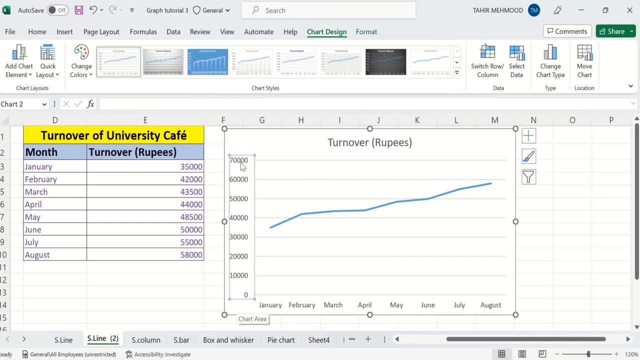 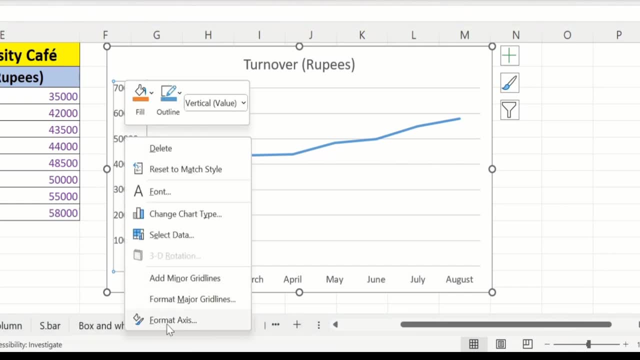 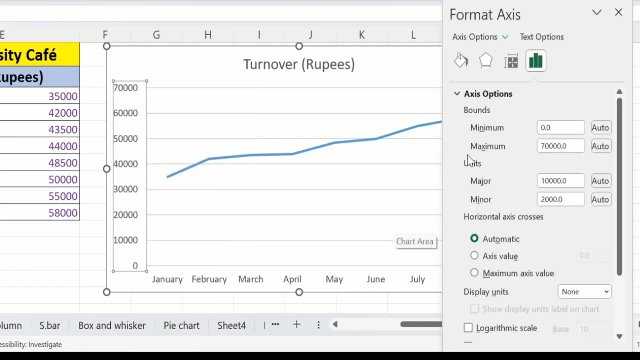 that you have selected the y-axis values. After doing that, place your cursor here, Right click, and you will find the option of format axis. Click on this option. Now, here under the banks, you will find the option of minimum and maximum values. I will 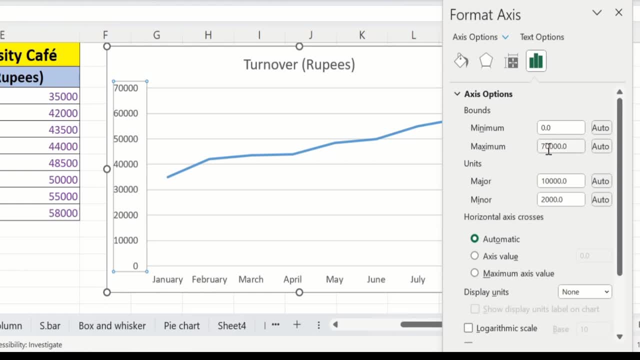 select 65000 instead of 70000.. After doing that, place your cursor anywhere in blank cell. You can see, here I have selected this one And here, under the bounds, you will find the option of minimum and maximum values. I will select 65000 instead of 70000.. After doing that, place your cursor anywhere in blank cell. 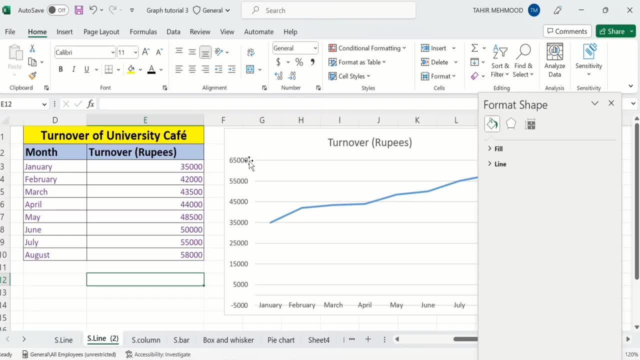 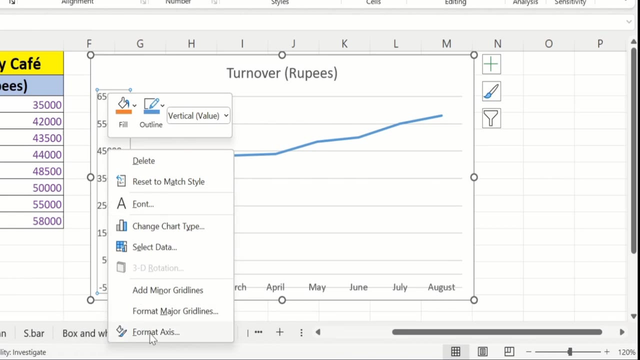 are changed from 70,000 to 65,000.. Similarly, you can also change the minimum values. For example, I want to change the minimum values to 25,000.. I will select this one. Right click Again, go to this format axis option And in format axis option you will find the minimum and maximum. 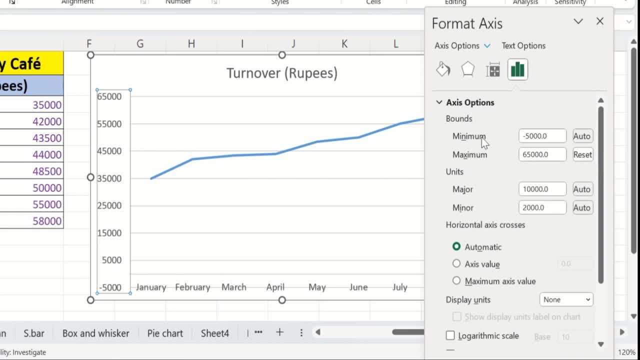 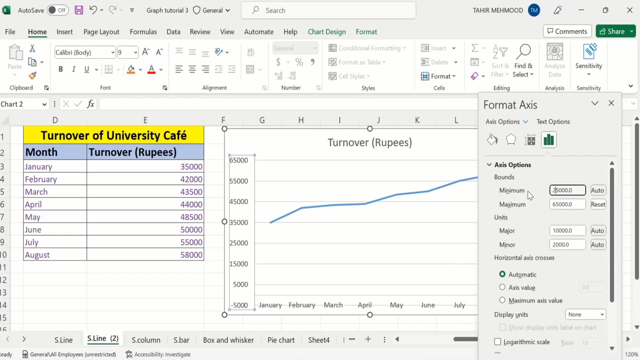 value. Currently you can see here, the minimum value is minus 5,000.. I will change it to 25,000.. After changing, click anywhere in sheet And you can see here the values is changed to 25,000.. 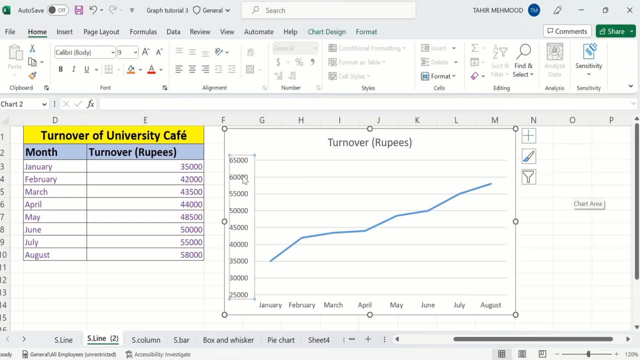 Now you will learn how to adjust the difference between these two values. Currently- you can see here- the difference between these two values is 25,000.. And you can see here, the difference between these two values is 5,000.. I will select this one Right click. Go to format axis option. 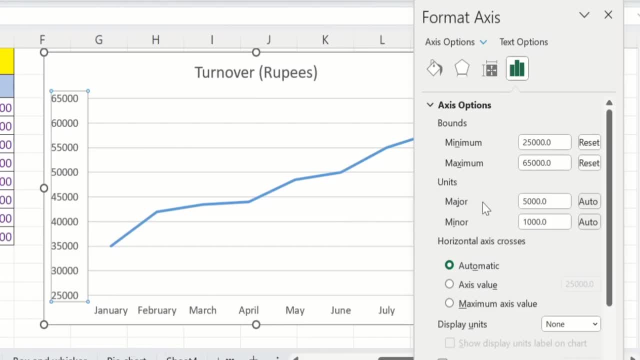 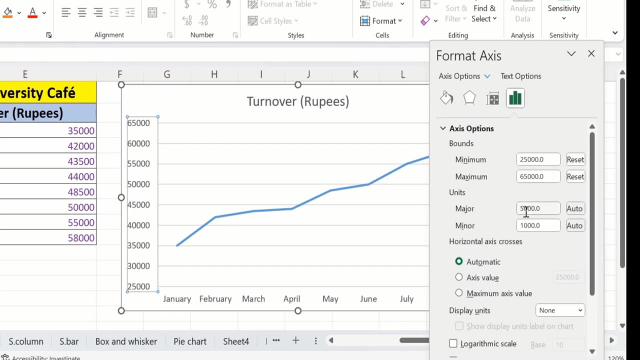 And under units- you can see here, the major and minor units option is there And in major units- you can see here- the difference is 5,000.. So Excel has displayed these values according to this difference, If I change it to 10,000,.